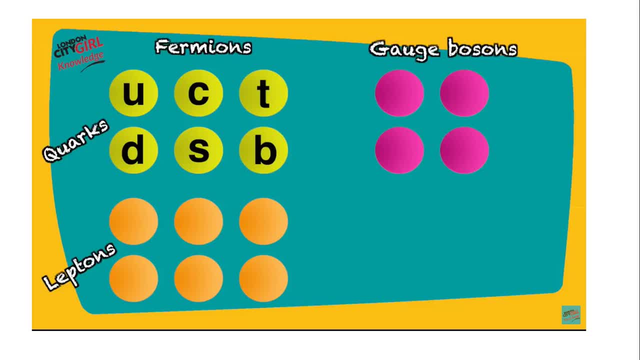 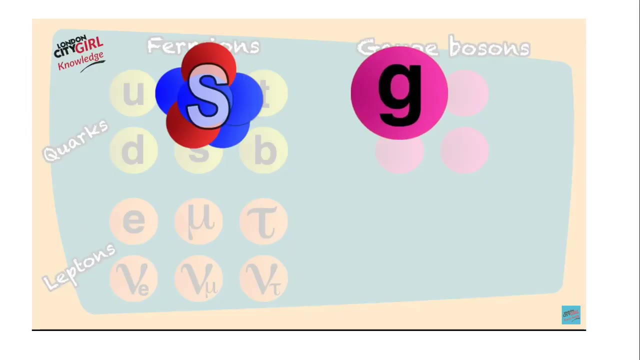 charm and strange top and bottom. There are six leptons: electron muon, tau electron neutrino, muon neutrino and tau neutrino. Fermions create matter and the gauge bosons carry the forces between the matter particles. Gluons mediate the strong force between the quarks holding them. 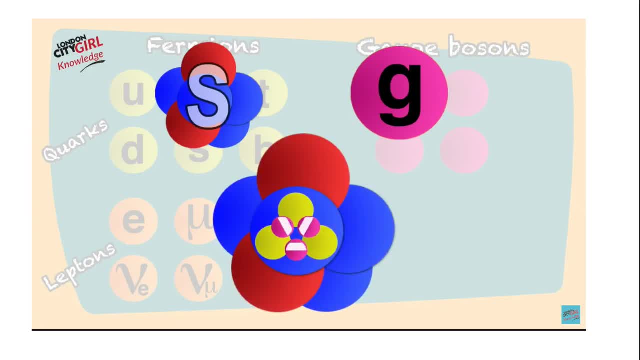 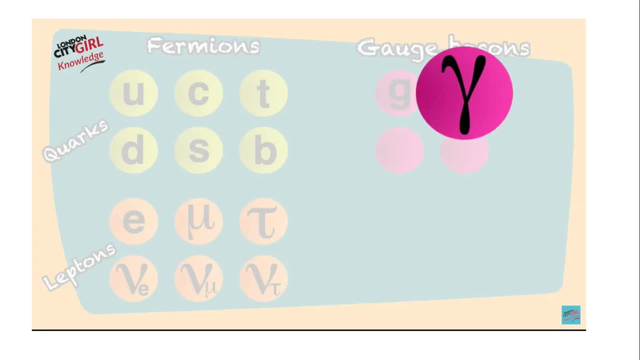 together within the protons and neutrons. Gluons also mediate the strong force between the protons and neutrons, holding them together within the nucleus of the atom. Photons are particles of light which carry the electromagnetic force that holds the electrons in atoms W and Z, bosons carry. 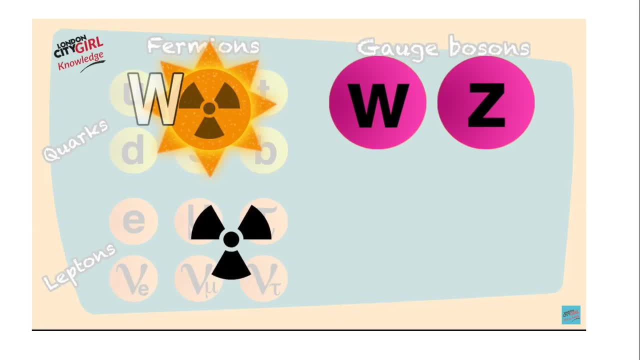 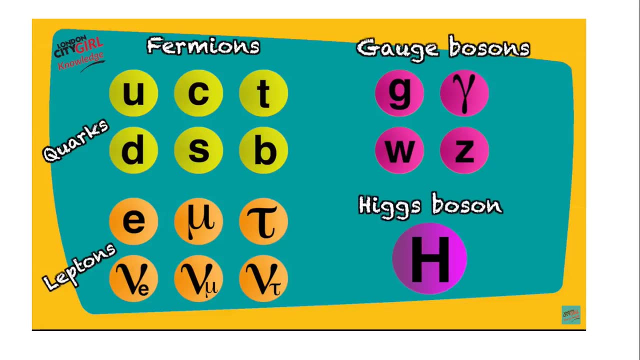 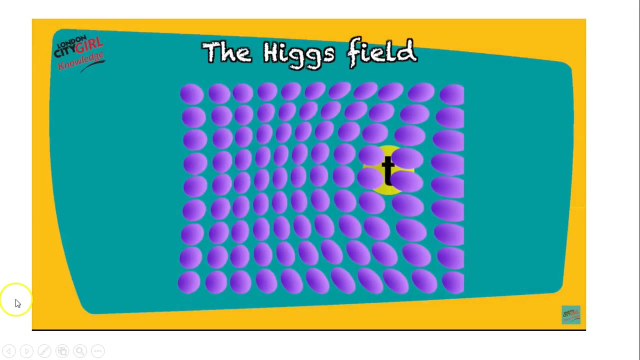 the weak nuclear force and they are involved in some forms of radioactivity and they play a role in how the stars burn. And finally, the Higgs boson is a corresponding carrier particle of the Higgs field, which is a quantum field that permeates all of space. Particle interactions with the Higgs. 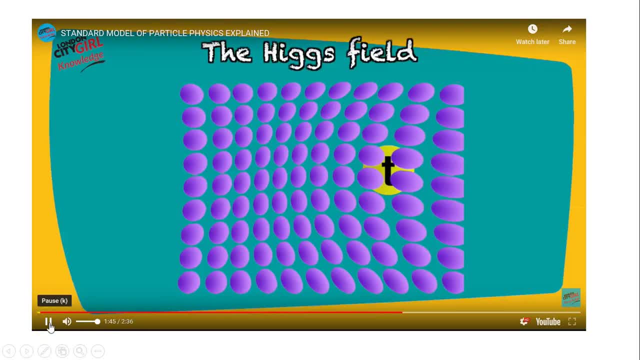 field are very important. The Higgs boson is a quantum field that permeates all of space. Particle interactions with the Higgs field impart particles with their mass and the Higgs boson is the local excitation of the Higgs field. If you like my content and want to help me make more, 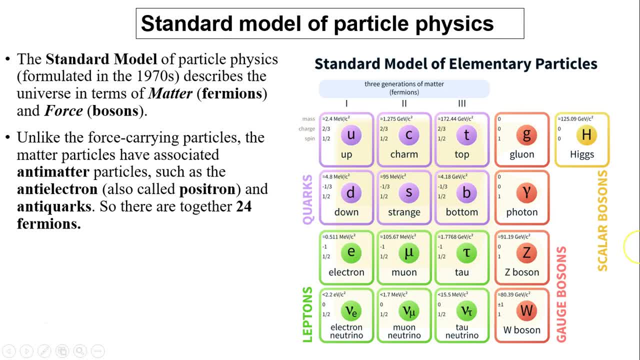 So the standard model of particle physics, including, describes the universe in terms of matter and force. So, unlike the force carrying particles, the matter particles have associated anti-matter particles, such as anti-electrons and anti-quarks. So there are 24 fermions. So fermions, these are matter particles. right over here, Up down charm. 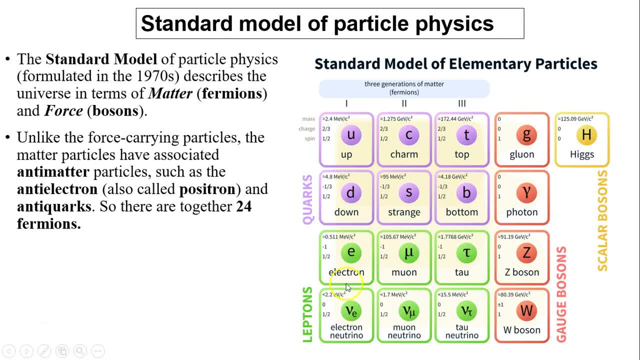 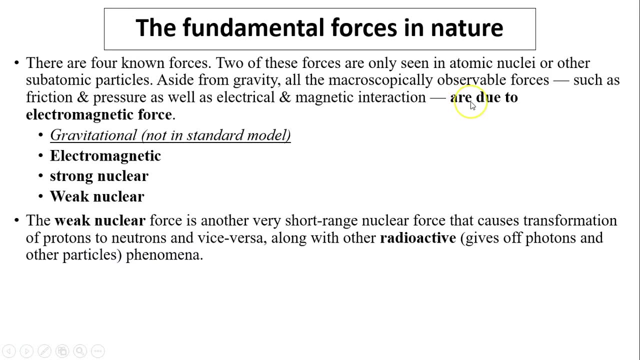 string, top and bottom. And here is the left hand: electron- mu and tau and electron neutrino, mu and neutrino and tau and neutrino. And here are the force carriers, or called bosons. So the force carrier is the is responsible for the forces between the particles. 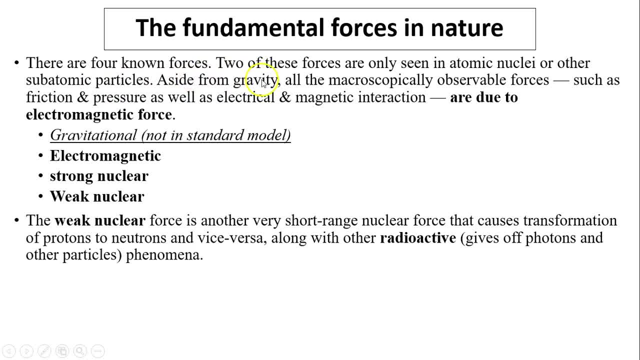 So there are four known forces. These are called fundamental forces. Two of these forces are only seen in atomic nuclei and other subatomic particles. They are strong nuclear force and weak nuclear force. Aside from gravity, all the microscopically observable forces, such as 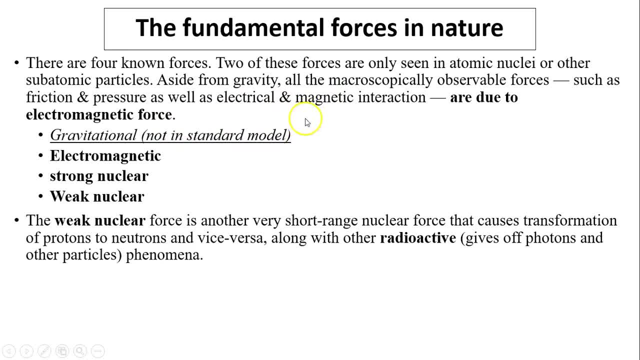 friction force or normal force. they are all the results of electromagnetic forces. So the four fundamental forces are gravitational force, electromagnetic force, strong nuclear force and weak nuclear force. By the way, in the standard model. gravitational force does not belong in the standard model. 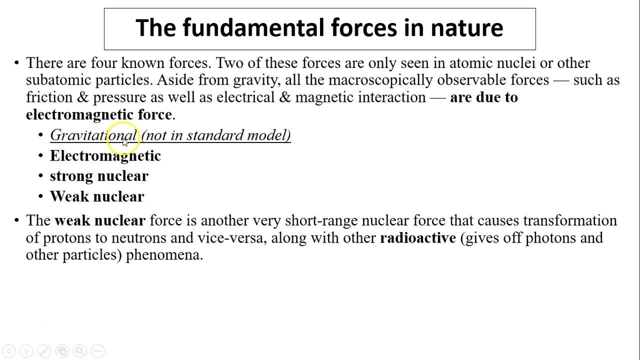 Only these three forces. Now, scientists are still working on gravitational force. Kant seems to work it out- Not yet. So the weak nuclear force is another very short-ranged force that we haven't talked about. That causes transformation of protons to neutrons and vice versa, along with other radioactives. 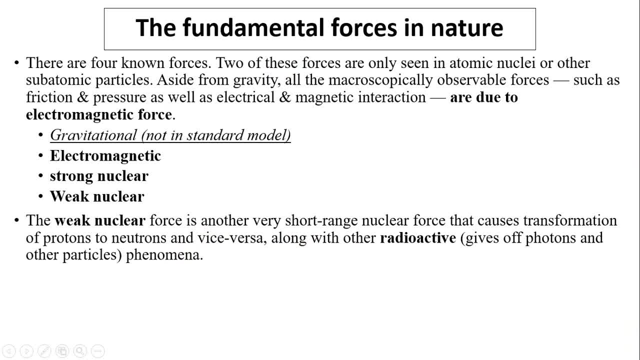 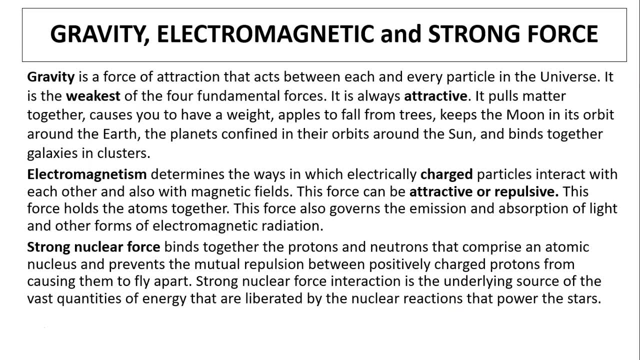 It gives photons and other particles, other radioactive phenomena. Now let's take a look at the three forces we have kind of learned Gravity: Gravity is a force of attraction that acts between each and every particle in the universe. It is the weakest of the 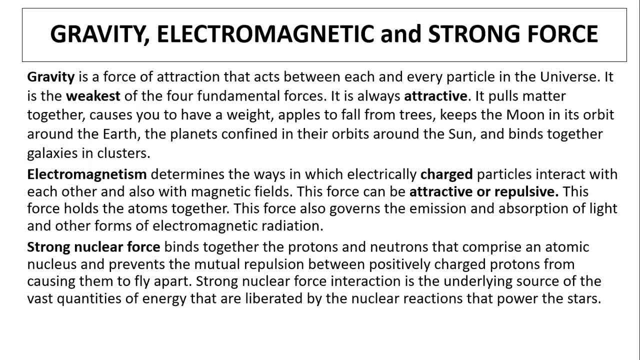 four fundamental forces. It is always attractive, It puts matters together, causes you to have a weight, apples to fall from the tree and keeps the moon on its orbit around Earth- The planets confine in their orbits around the sun- and binds together. 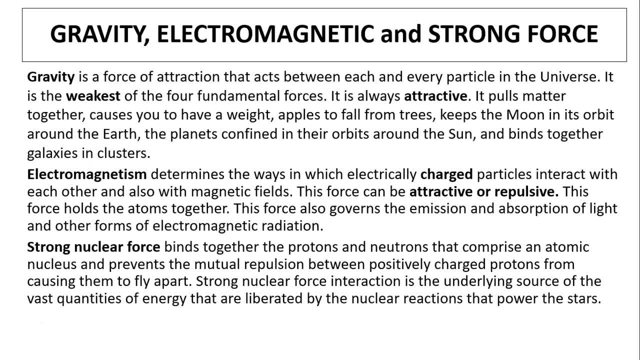 galaxies in clusters. Electromagnetism or electromagnetic force, determines the way in which electrically charged particles interact with each other and also with magnetic fields. This force can be attractive or repulsive. This force holds the atoms together. This force also governs the emission and absorption of light and 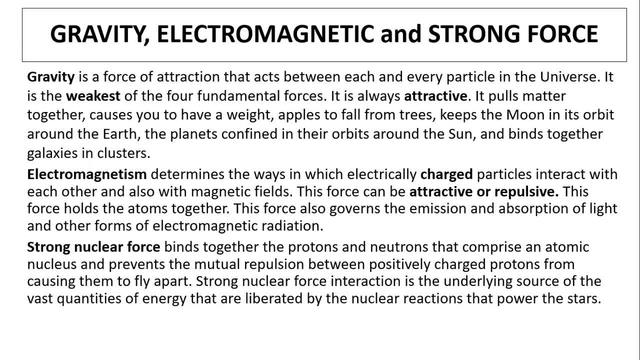 other forms of electromagnetic radiation. The strong nuclear force actually binds together the protons and neutrons that comprise atomic nucleus and prevents mutual repulsion between positively charged protons from causing them to fly apart. Strong nuclear force interaction is the underlying source of vast quantities of energy. 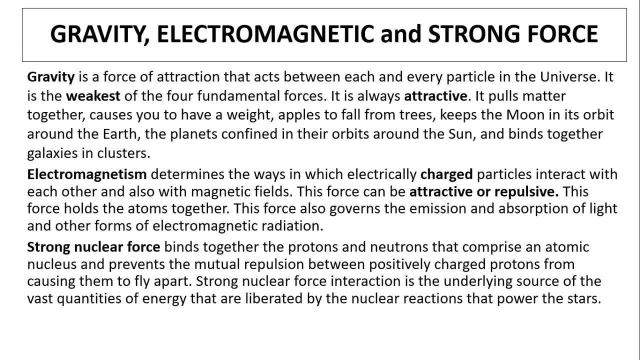 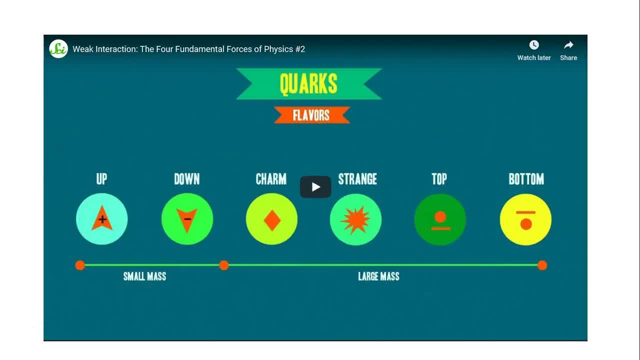 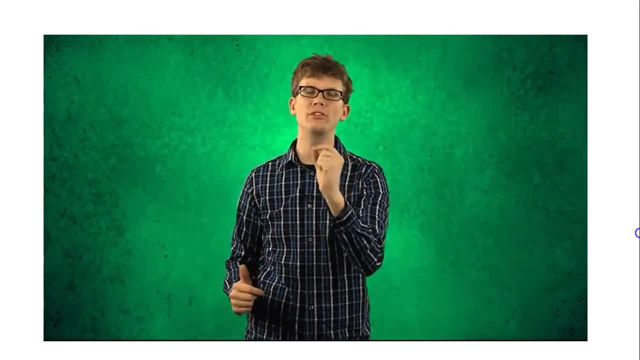 that are liberated by nuclear reaction that powers the stars. So one more force is the weak nuclear force that we haven't talked about. Let's take a look at a series on the four fundamental forces of physics, A mere four forces that make the whole universe work. 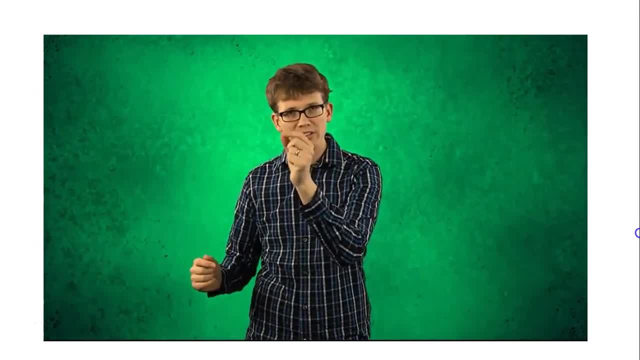 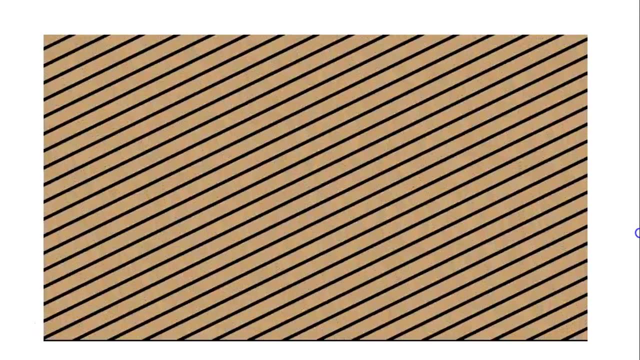 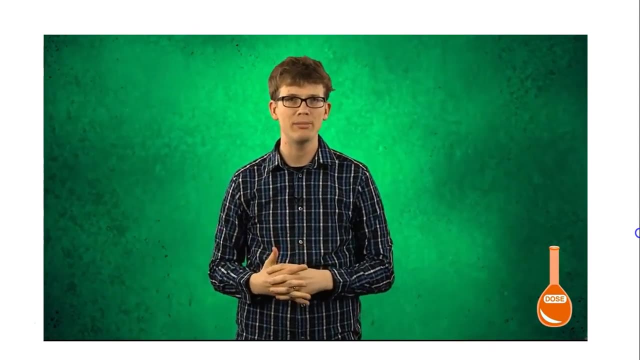 And in this installment we're talking about a force that acts over very, very teeny, tiny distances: the weak force. Without it, the sun would not shine, we would not have elements like radium or plutonium and we wouldn't have carbon-14 dating. 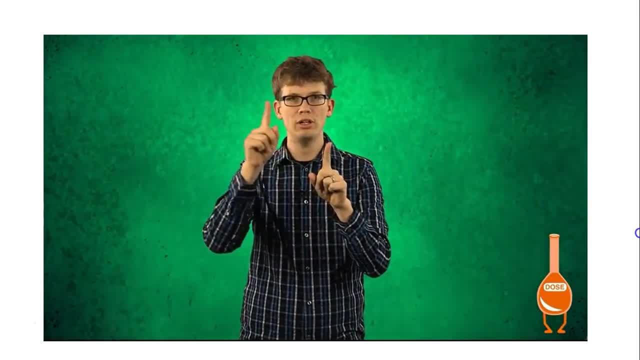 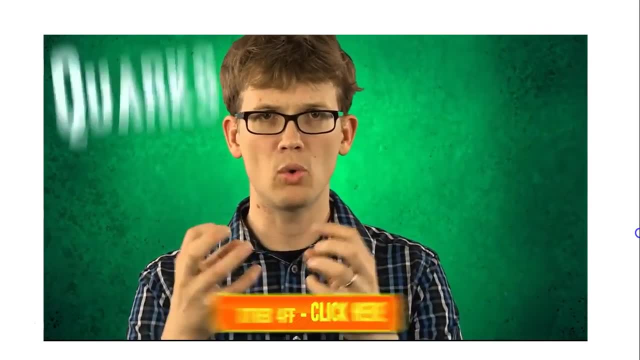 All of these things require one particle to turn into another particle through particle decay. Remember strong force. It acts on a proton or a neutron to hold its component, quarks, together, And one way that we describe quarks is by their color. It's just a characteristic. 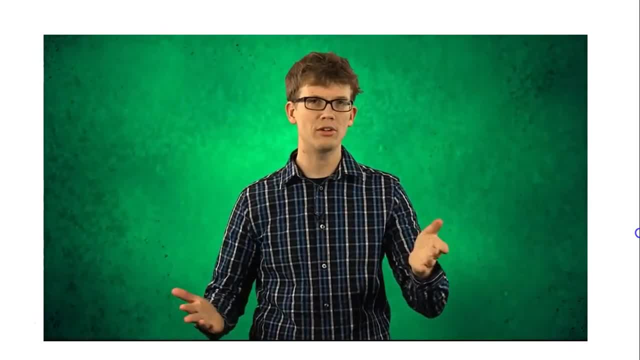 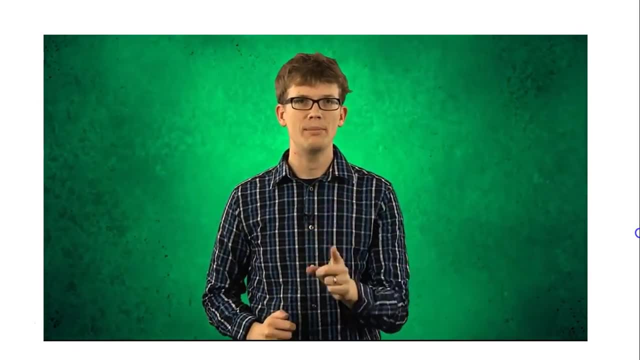 of a quark, sort of like a charge, is a characteristic of an electron. Weak force acts on quarks just like strong force does, but instead of changing its color, it changes its flavor. There are six flavors of quarks: lemon-lime, root beer, hazelnut. 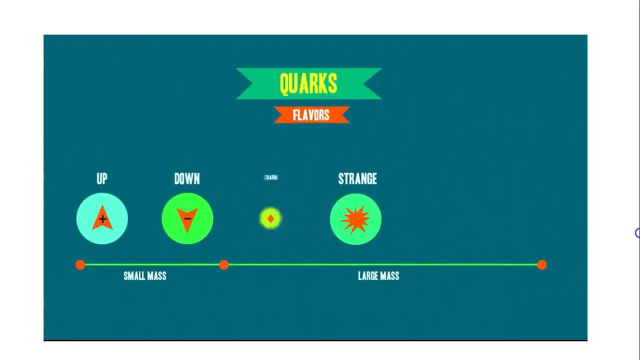 sorry, Seriously, you've heard of these. uh, up down, strange charm. top and bottom. Up quarks have a slight positive charge, while down quarks have a slight negative charge and they both have the smallest masses of all the quarks. The other quarks have charges too, but they're all much heavier. 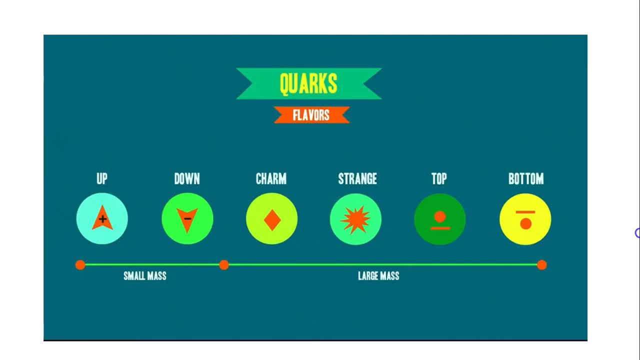 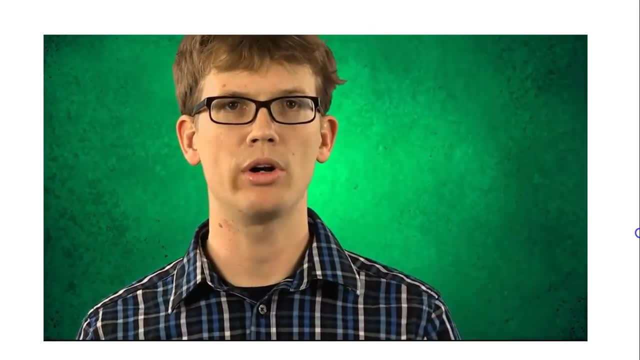 and much rarer, because they quickly decay into up and down quarks. Up and down quarks are what most stuff is made of. Neutrons are made up of one up quark and two down quarks, while protons are two ups and one down. Now the weak force. 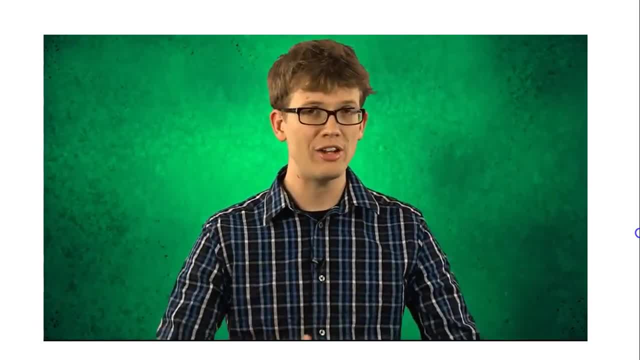 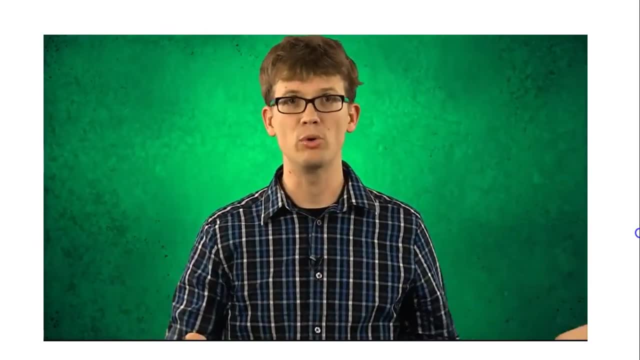 changes quark flavor. So when a quark inside of a particle changes, that changes the whole identity of the particle. This is crazy stuff to me to think that you can actually like, just through this force, change a proton into a neutron. 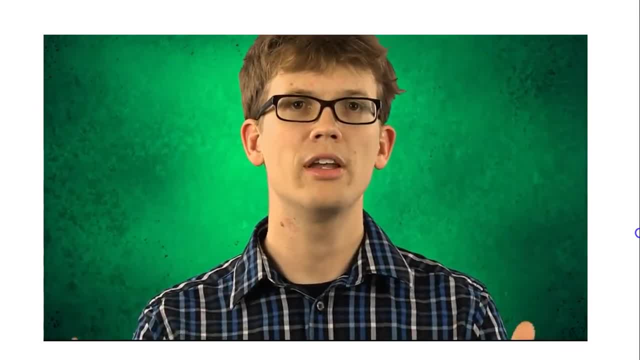 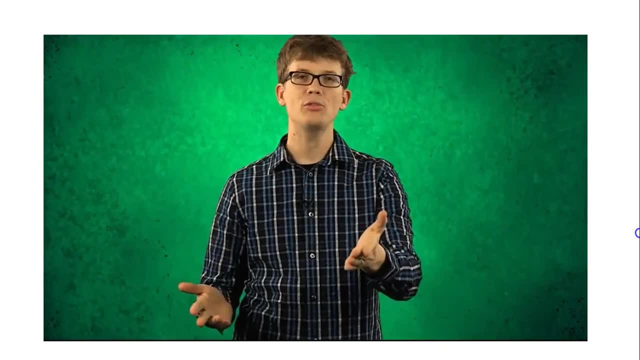 It's nuts, In addition to quarks, and thus neutrons and protons. weak force can also interact in a similar way with leptons, the most famous of which is the electron, but also including neutrinos, And as with all fundamental forces. 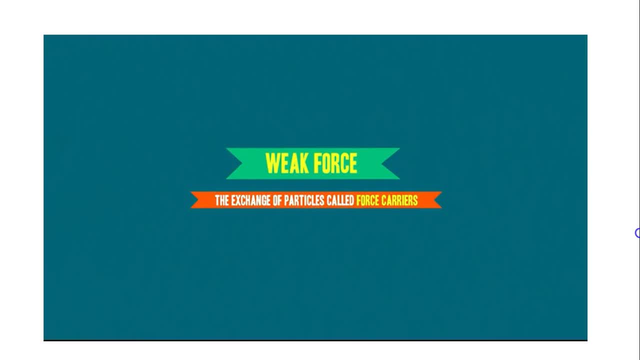 the weak force involves an exchange of particles called force carriers, which are these weird, barely existing particles that convey forces between other particles. Weak force has two force carriers: the W-bosons, which can be either positively or negatively charged, or the Z-bosons, which have no charge. Now let's watch some weak. 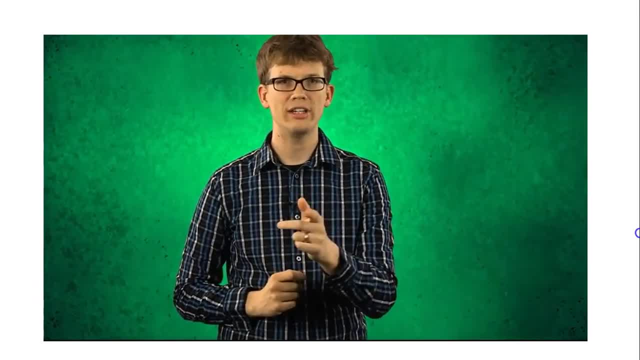 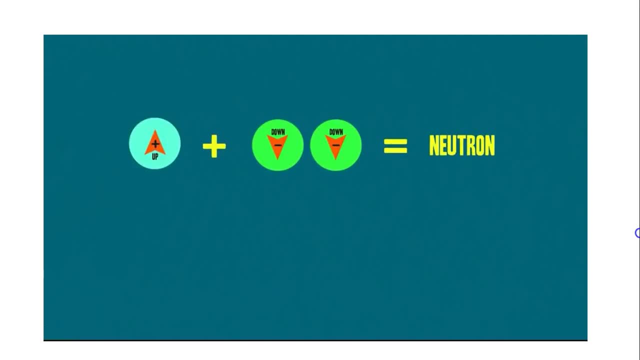 interaction at work. How about we make a neutron change or decay into a proton? To do this we're going to need a neutrino passing by. So remember neutrons are one up- quark- and two down. quarks and protons are two. 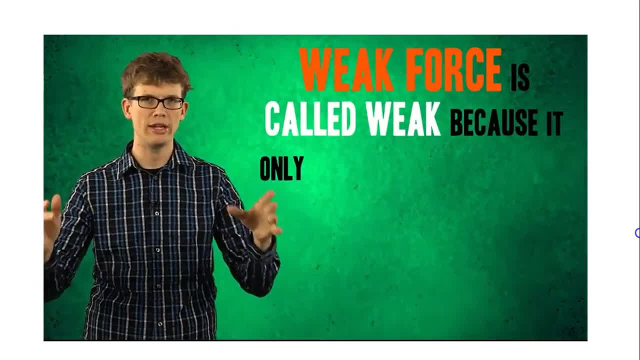 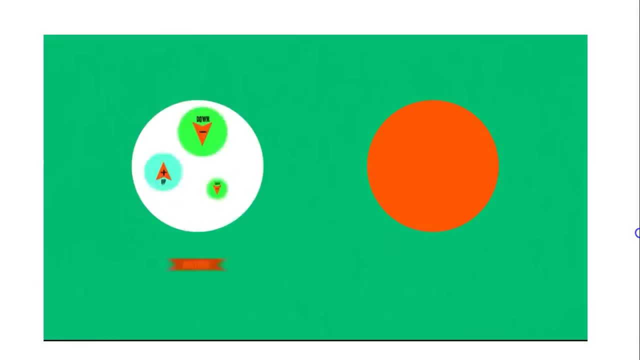 up quarks and one down quark. The weak force is called weak because it only operates within a teeny, tiny, tiny, tiny range, about 0.1% of the diameter of a proton. So say, our neutron comes close enough to a neutrino. 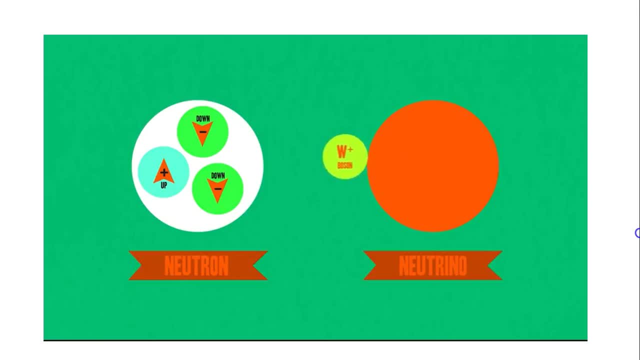 A positively charged W boson would travel from the neutrino to that neutron. That's the weak force right there. The neutrino having lost a positive boson, becomes negatively charged, turning it into an electron And over on the neutron. meanwhile, the positive W boson encounters a down quark. 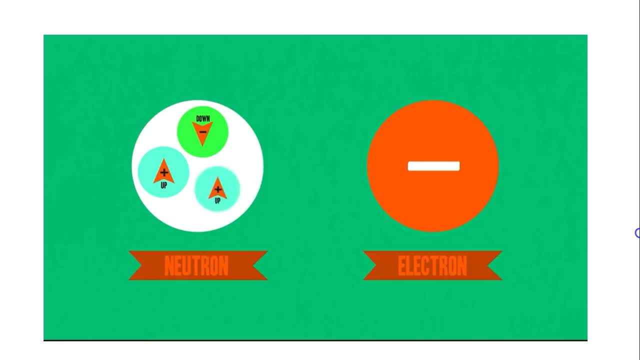 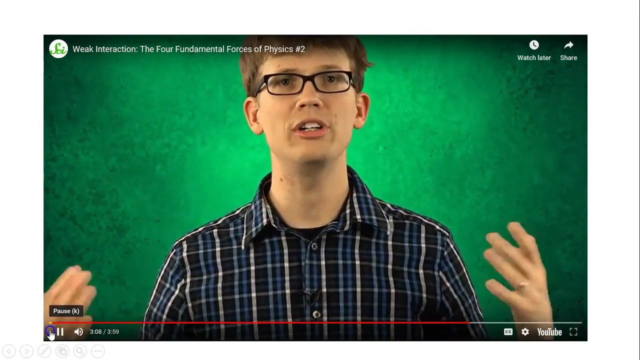 and changes its charge from slightly negative to slightly positive. And since neutrons and protons have a difference of just one quark flavor, this changes the neutron into a proton, With the composition of the nucleus that contained this neutron having changed, the atom itself has changed too into an entirely new element. 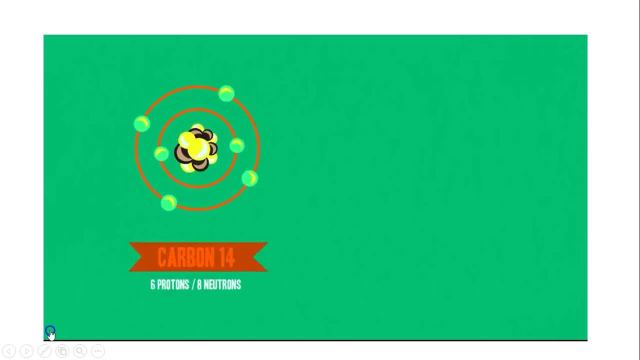 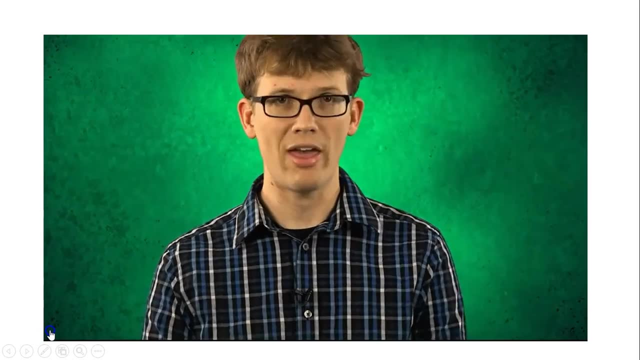 If this was a carbon-14 atom with six protons and eight neutrons, through the weak force it just decayed into a nitrogen-14 atom with seven protons and seven neutrons. And that actually happens. It happens all the time. 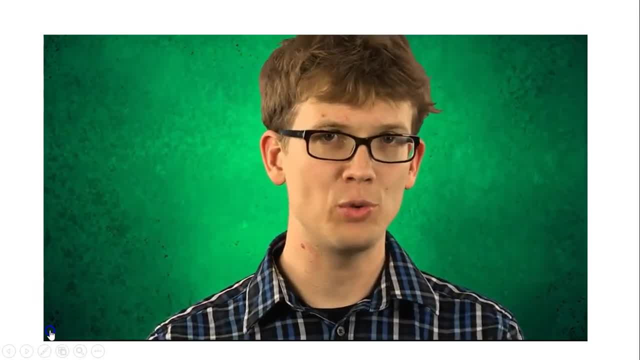 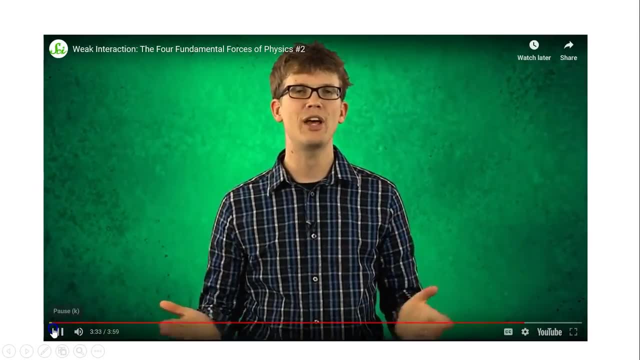 And it's how carbon-14 dating works. So there it is. The weak force is actually able to change the identity of particles when they come very, very, very, very, very close to each other. Thank you for watching this episode of SciShow. 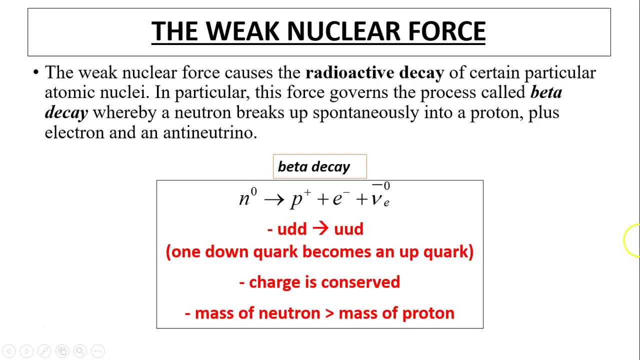 If you would like to know more about the f-. Okay, so the weak nuclear force. The weak nuclear force causes the radioactive decay of a certain particular atomic nuclei. As you saw, it's a carbon-14 dating. So in particular, this force governs the process called beta decay. 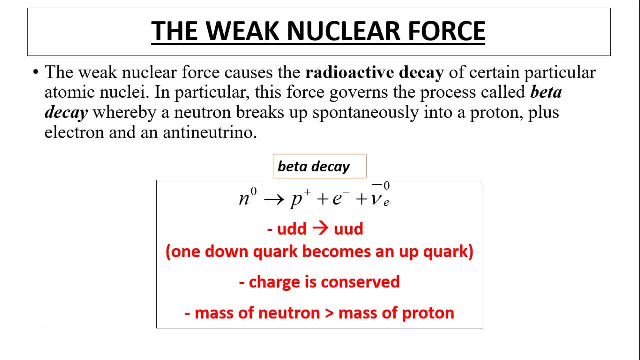 where a neutron breaks up spontaneously into a proton plus electron anti-neutrino. So here is again the equation for beta decay. We did this before in the last video. So neutron is up, down down. This up down down changed to a proton, which is up up down. 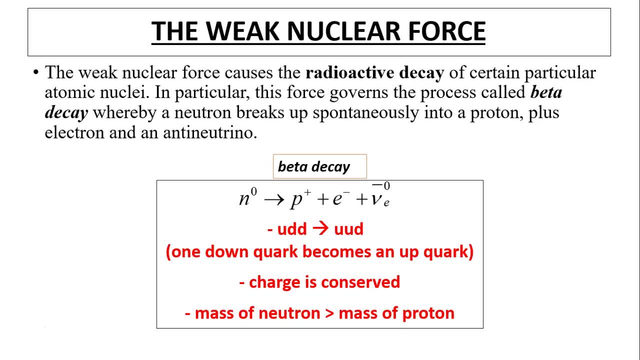 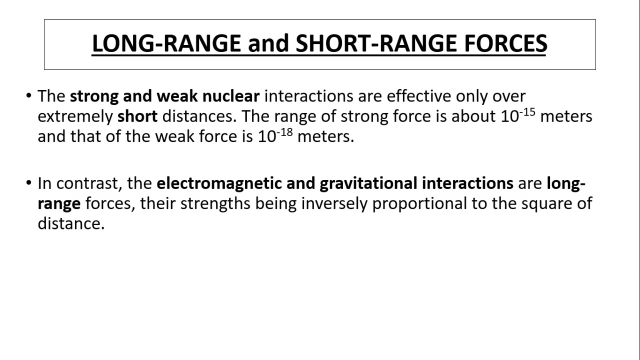 So one down quark basically changed to an up quark. So charge is conserved and the mass of the neutrino, mass of a neutron, is bigger than mass of proton. in in this conversion, in this beta decay, now all the forces can be categorized into long-range force or short-range force. 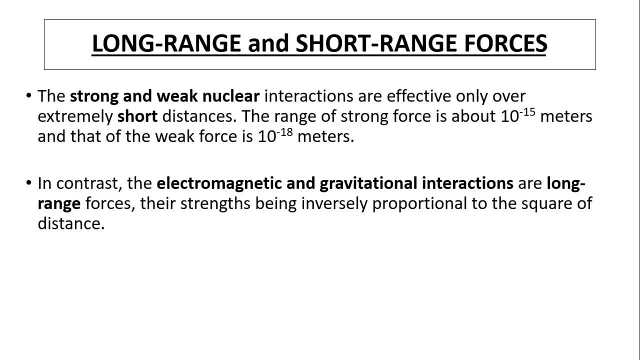 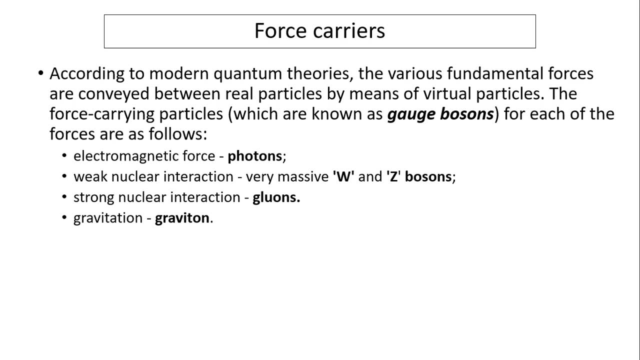 both strong and weak. nuclear force that happens inside a nucleus, so they are very short-range force. in contrast, electromagnetic and gravitational, those are long-range forces, force carriers. so we know the um bosons are force carriers and they are a kind of communicating between the particles and the community, communicating the force between them. 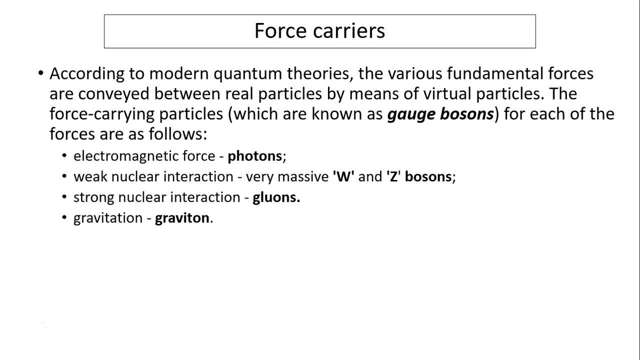 so, according to modern quantum theories, the various fundamental forces are conveyed between real particles by means of virtual particles. the force carrier particles, which are known as age bosons for each of the forces are as follows: electromagnetic, that's called photon. we use gamma for to represent that a weak nuclear interaction. w and z boson. 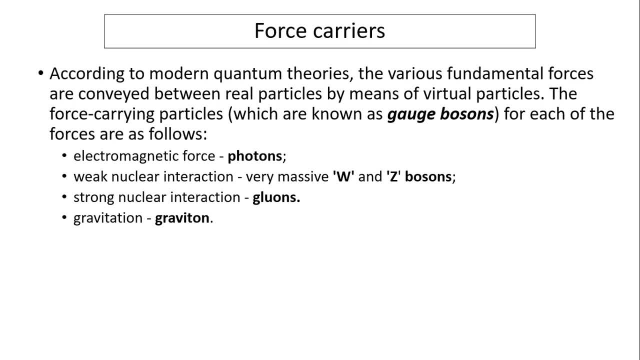 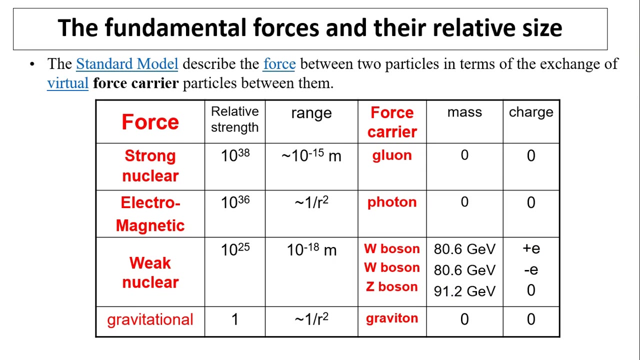 and strong nuclear force: we use gluon. and gravitation- we use graviton. this is why the gravity doesn't belong to uh. this uh standard um model is because people cannot, uh we haven't found a graviton to select Anna and include one more thing: um, radiation is more like a large particle. 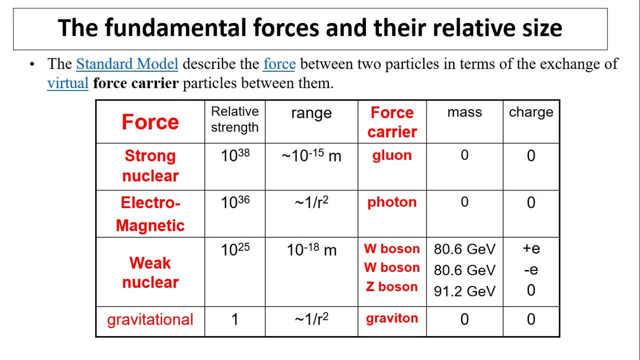 so we can and use擊 to represent that. a strong nuclear force and the relative strength. next one, the fundamental forces and their relative size. so standard model describe forces between particles in terms of exchange of virtual force carriers between them. so here are the forces. strong nuclear force has the relative strength 10 to the 38 if we consider. 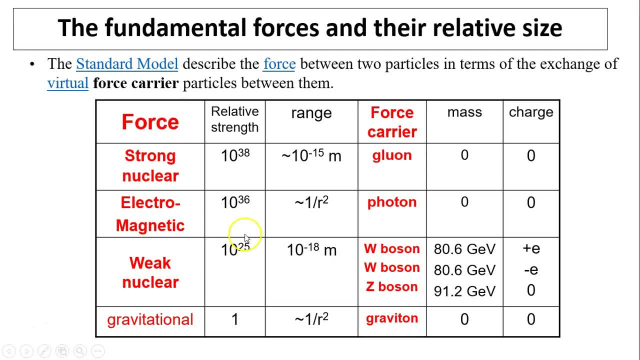 gravitational is one. so this 10 to the 38 times weak nuclear force is 10 to the 25. they are all very big range. the smallest range we said a nuclear force weak nuclear force is very, very uh is weak is because the range is very, very small. 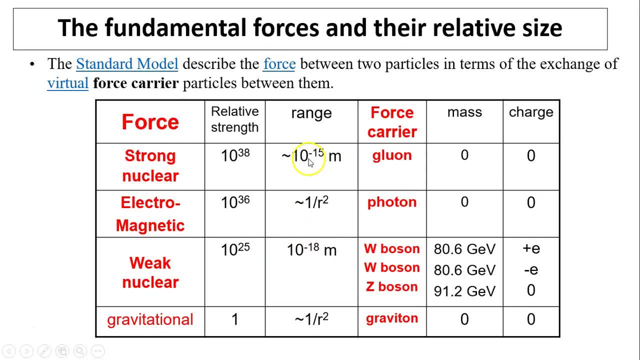 and here is strong um. nuclear force is range of 10 to the 50 meters, but weak nuclear force is 10 to negative 80 meters. here are the uh, relative uh, the force carrier, carriers glulian for strong nuclear electromagnetic is photon and weak force is w boss on c bosa.